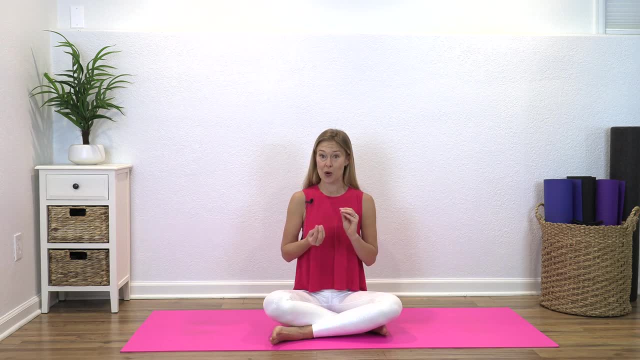 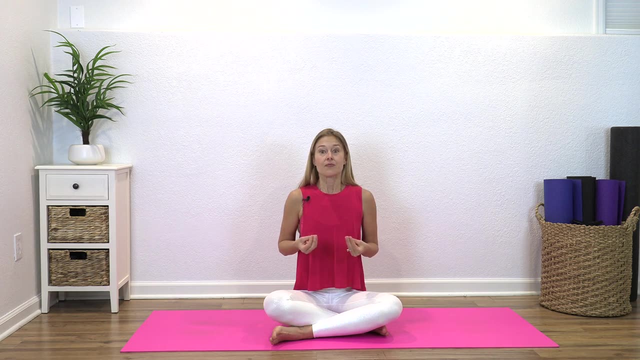 the anatomy as well. I'm going to use the words of what we're working and just work with me here. I want you to think about taking a deep breath in and then exhale On the next one. We're going to contract on the exhale. What I want you to think about is that you are 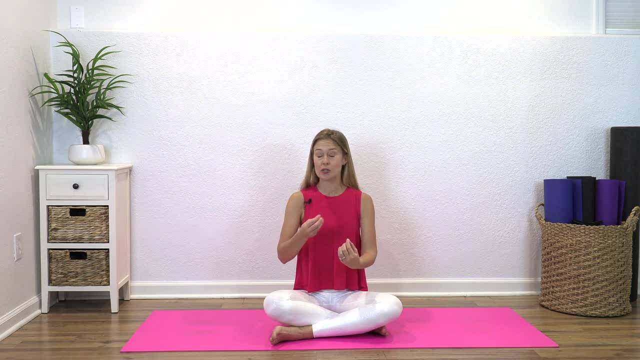 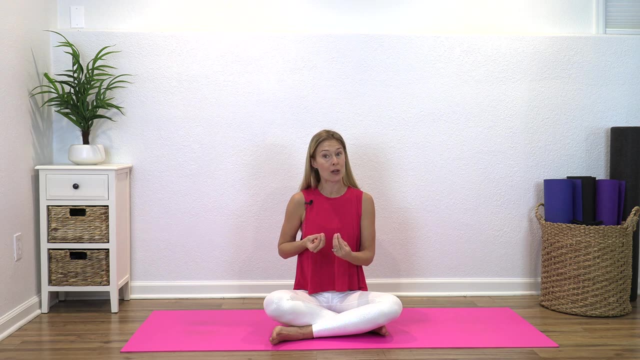 drawing your pubic bone back towards your vagina When you exhale. that's what you're thinking about doing. Draw your pubic bone in the front here, back towards your vagina. Take an inhale, exhale, pull it in. Good job, Inhale, relax. That's just as important You. 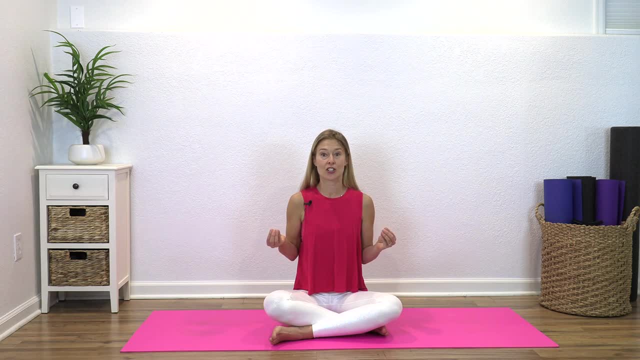 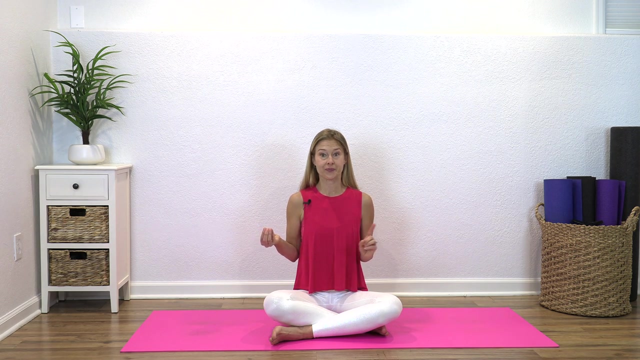 inhale, relax Exhale, draw it in again. You want to try to hold it for the full exhale and then you're going to inhale and relax. Do one more Inhale, exhale, draw it in and. 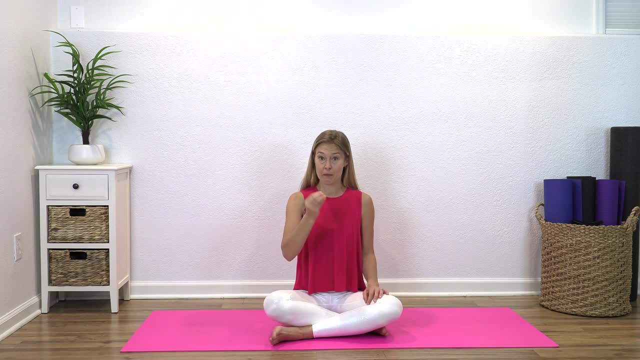 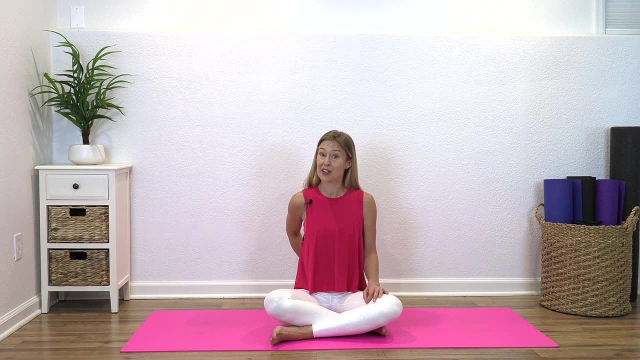 then relax. Now that was the front part of the pelvic floor musculature. We need to work the back part as well. I want you to think about your tailbone. If it helps, you can think about your anus. That's where we're working is back there. Take an inhale, exhale. 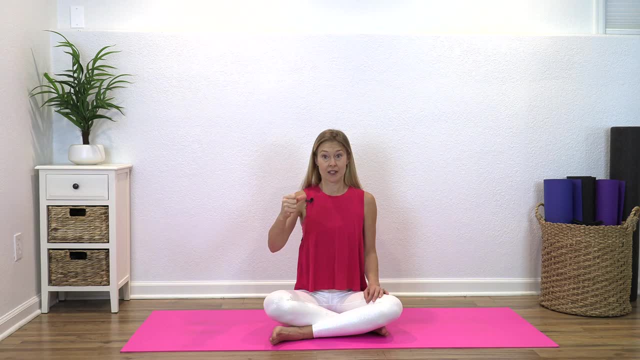 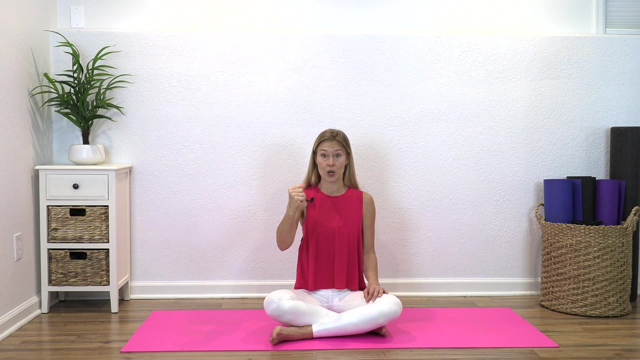 Now draw from your tailbone towards your vagina, Then inhale, relax. That should feel just a little bit different. You relax on your inhale, Exhale, gently, draw it in. Now we're going from the back forward. If this doesn't make sense to you yet, that's okay. I just 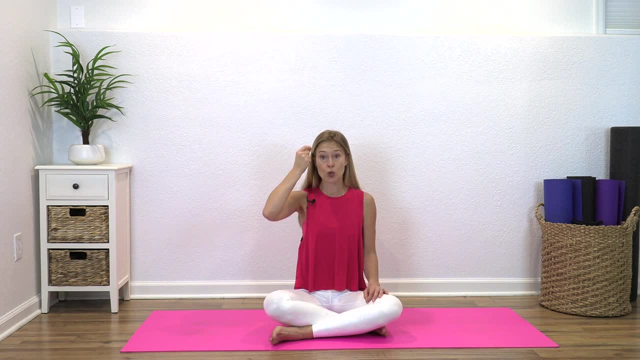 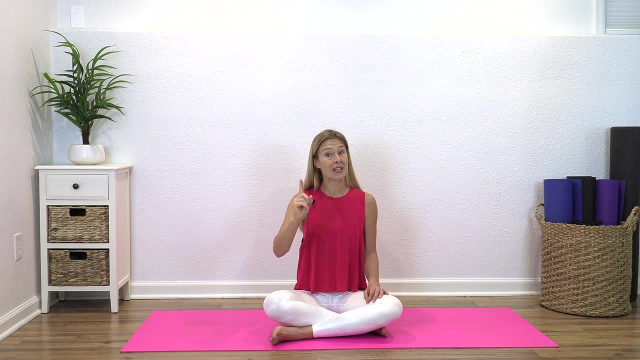 want you to keep practicing, keep practicing, keep practicing. We are slowly building the muscle connection from your brain to the musculature. Now, final piece to this. Don't skip this part. What you're going to do is draw them both in and 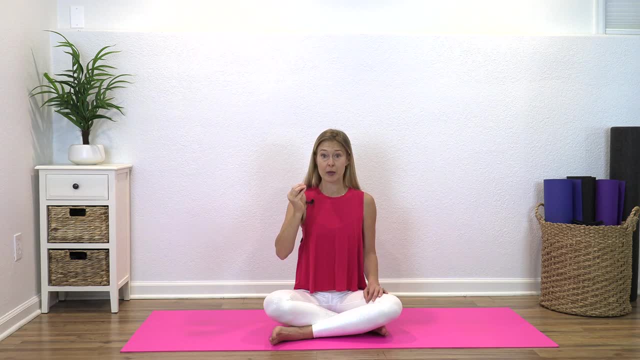 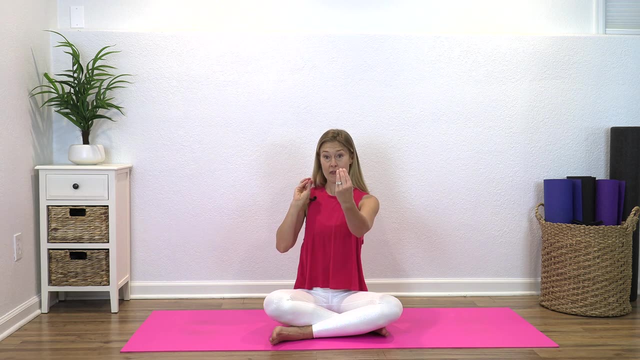 up at the same time. A good cue that works for a lot of people is: you're going to think about sitting on a bean, a dried bean. What we're going to do is pull from the front and the back at the same time, and then you're going to pull that bean up into your vagina. 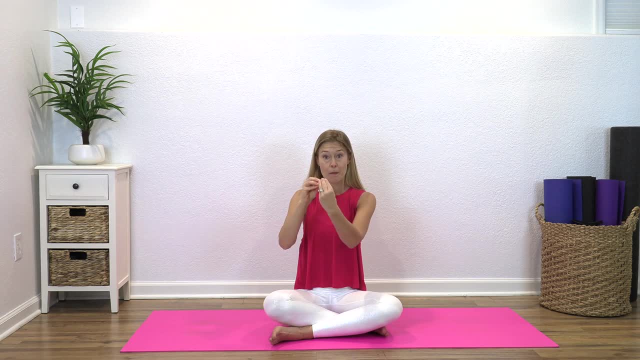 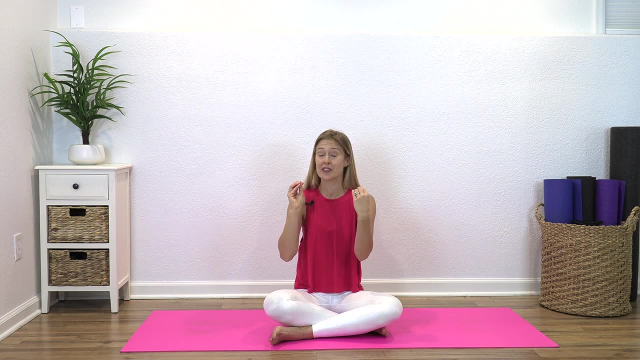 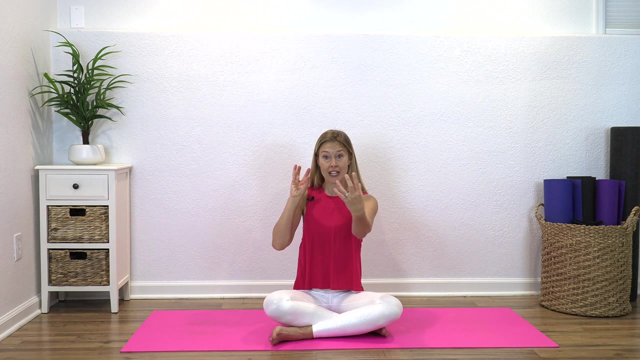 If it helps, you can think about sitting on a Kleenex and trying to pull that up and in and then you relax and let it back out. I know it might sound silly, You can laugh. if you want, Go ahead. These cues work. Inhale and exhale. Go ahead and draw it in again. 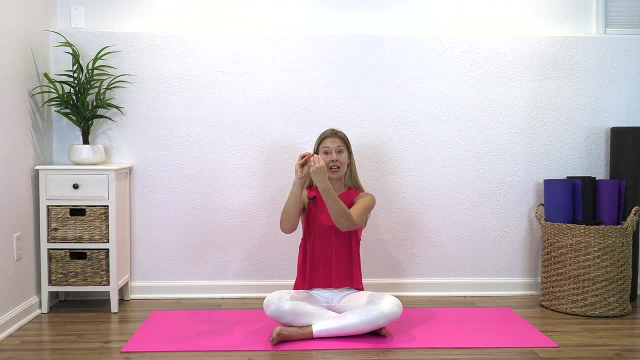 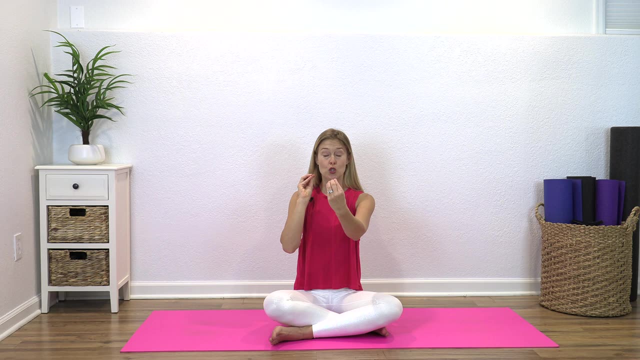 from front to back and then pull it up, Gently. pull that bean or that Kleenex up into your vagina and then you relax it back out. Do a few here as I'm doing this, I'm going to talk to you. You relax on the inhale, exhale, draw it in, pull it up, Continue to pull and 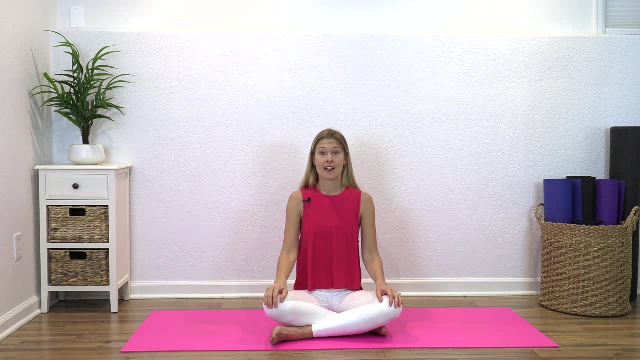 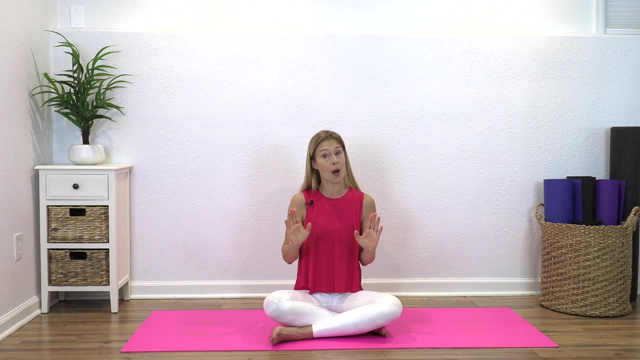 hold for that full exhale and then relax when you're ready. This is much more effective than a typical Kegel exercise. That idea of stopping the flow of urine- it doesn't work. Research actually shows us that when women use that cue, they're not contracting the. 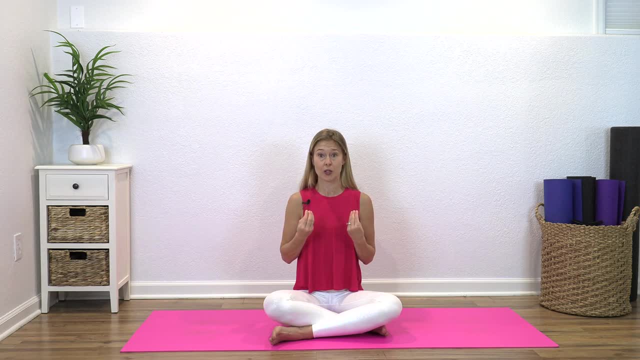 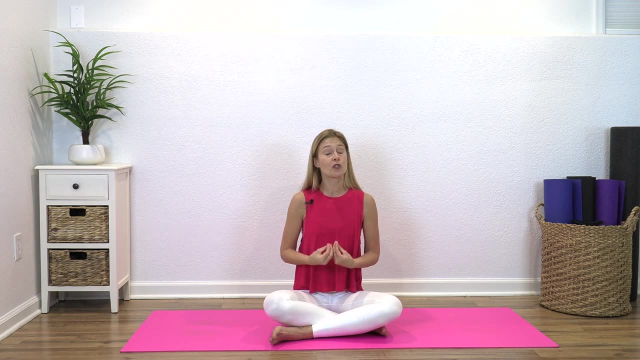 right muscles. I want you to really work and practice on this one. If you are in a place that you are really trying to work and build your pelvic floor muscles, then you need to do 50 of these a day. Keep coming back here to see me, if you need to, at least for 30 days. 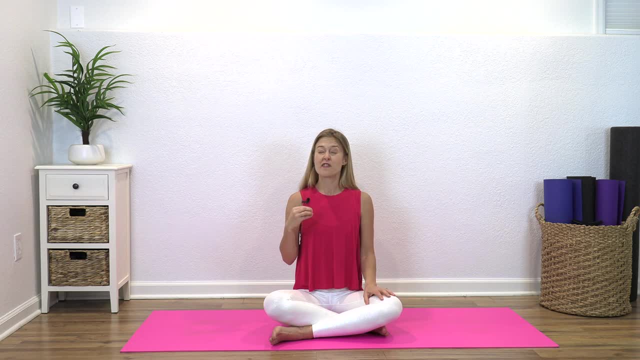 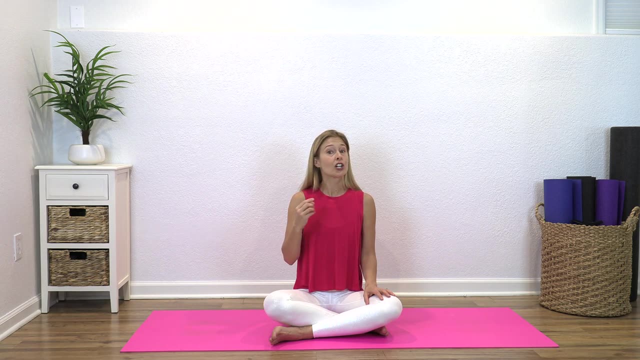 That's your homework: to do this video for 30 days. every day You're going to do 50 of these a day. You can do them laying down in bed. You can do them sitting in the car, sitting at your desk. You can do them laying on your stomach reading books to your kids. That's. 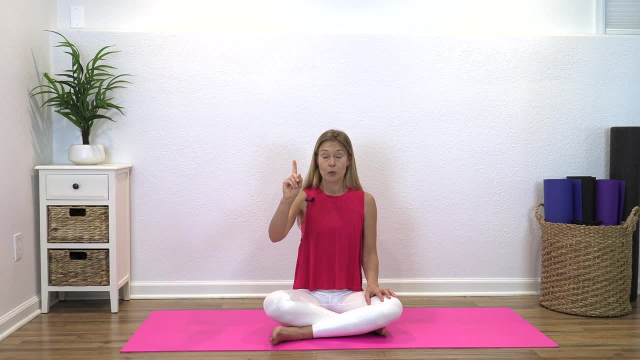 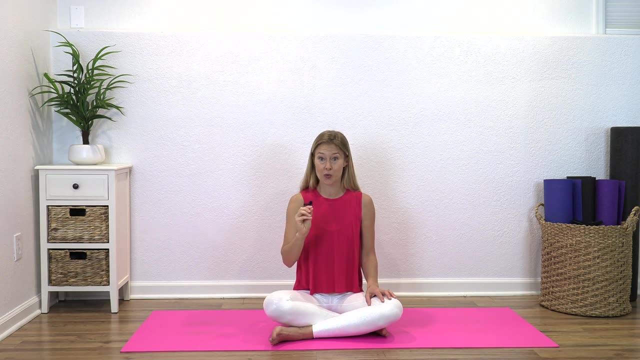 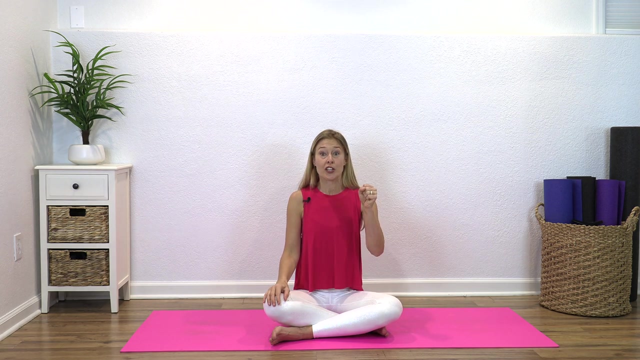 what I do half the time. Just make sure you do them. That's homework one, Homework two a day. Now we need to work fast: twitch fibers in the same area. This is what that means. You're going to take an inhale, Exhale. You are going to do five of those contractions as quick. 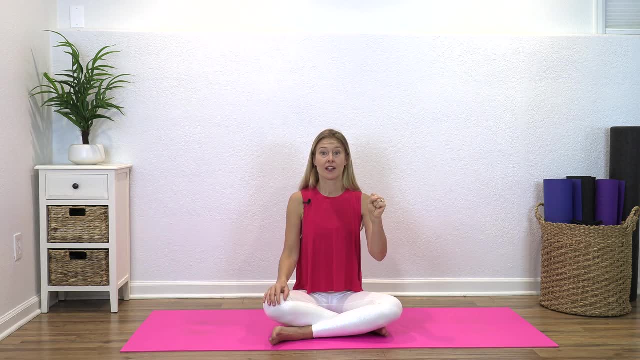 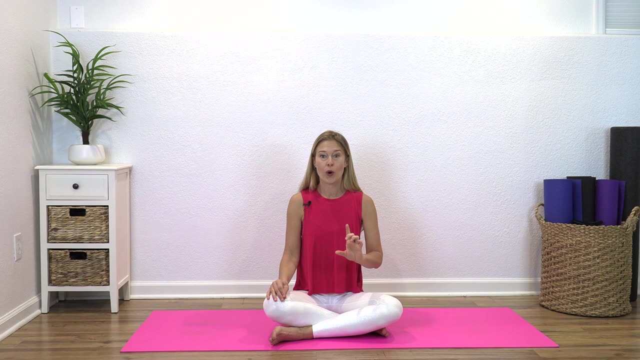 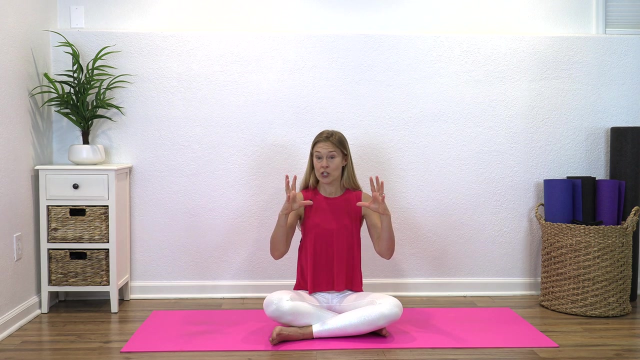 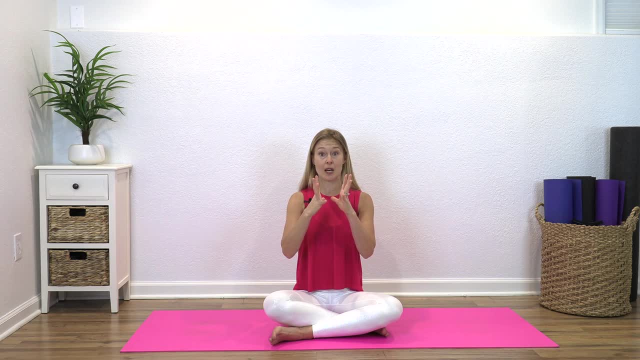 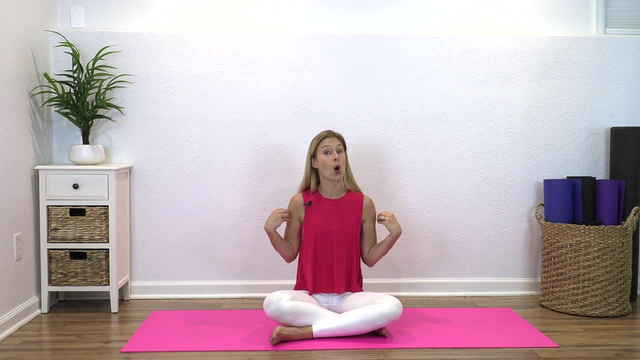 just did That, That contraction, right. You pull it in and up. so you suck that bean in and up. Relax the whole thing. Do it again right away. Relax the whole thing. You're trying, though, not to tense all the other muscles in your body when you do it. It's just as important to 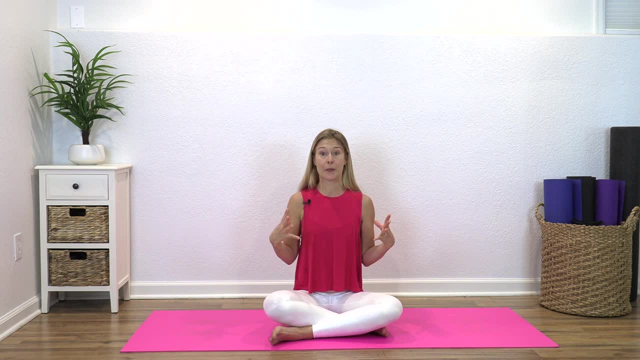 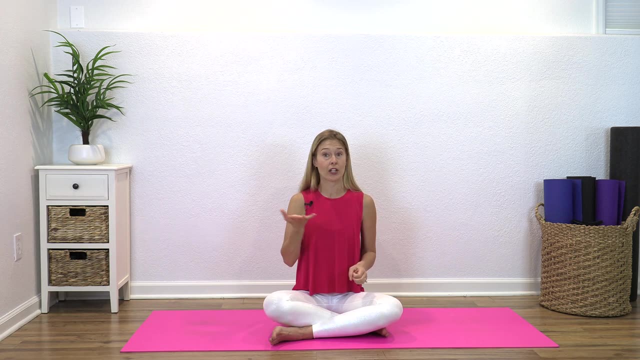 learn to relax, as it is to tighten. The difference is doing. those long, sustained contractions are going to help your pelvic floor during regular activity during the day. These quick ones that's going to help your pelvic floor during regular activity during the day, These 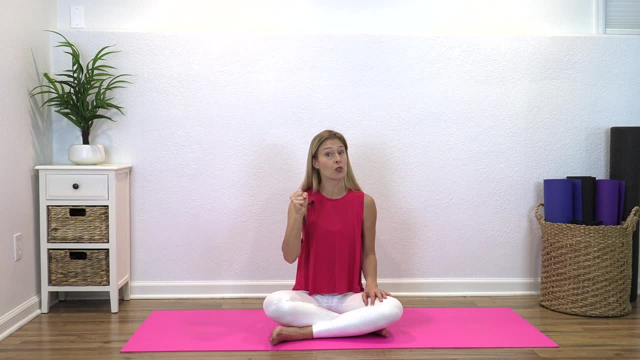 can help, like your incontinence. so if you leak urine a little bit when you jump, when you run, That's what this helps with, alright, And I want you to try to do 50 of those during the day. If it sounds like a lot, I know, Just do as many as you can. okay, I promise it. 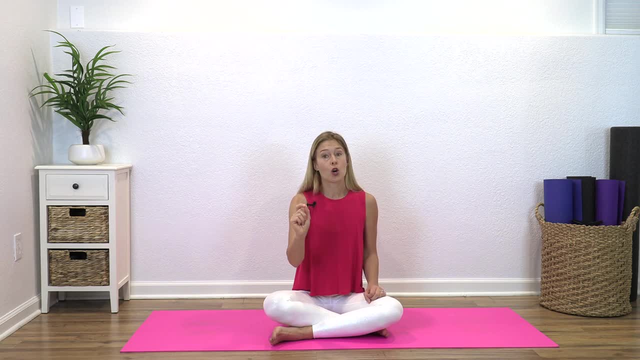 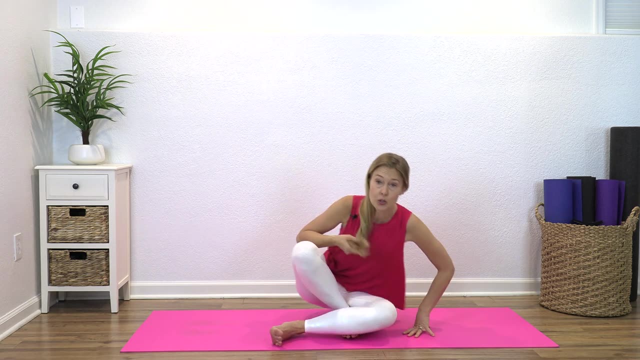 will make a difference. all right, So we're going to move on to homework. number two: That, Now that you understand those two different pelvic floor contractions that are really important. The next thing- and you might think this has nothing to do with your pelvic floor. 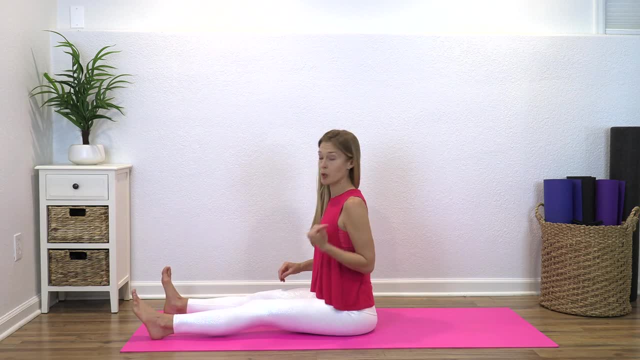 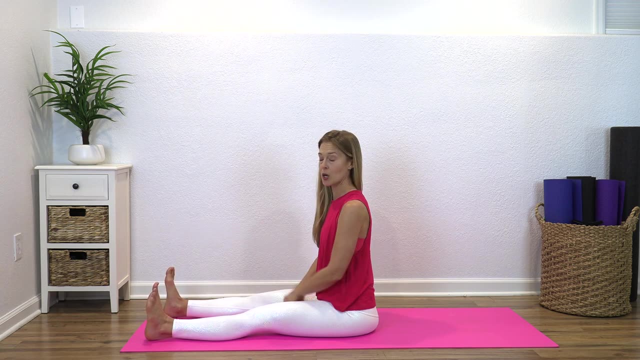 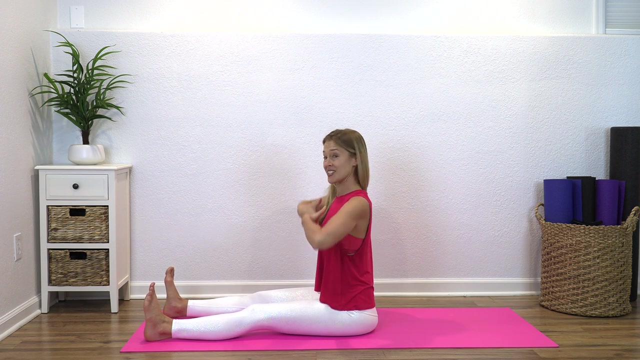 I promise you it does, and it's super important. sit with your legs out in front of you, have your legs about mat distance or shoulder distance apart. pull your toes back towards you. so what happens when the pelvic floor has a dysfunction is we also tend to lose all this space up in our abdominal canister and we lose 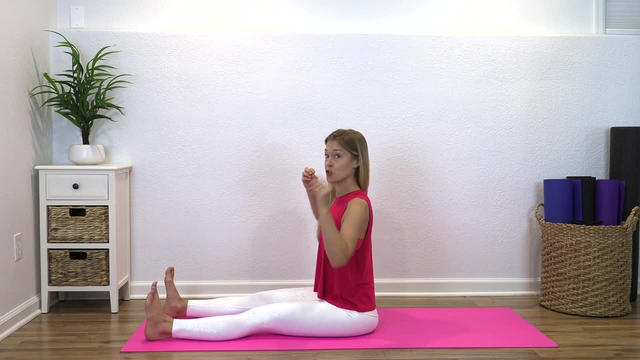 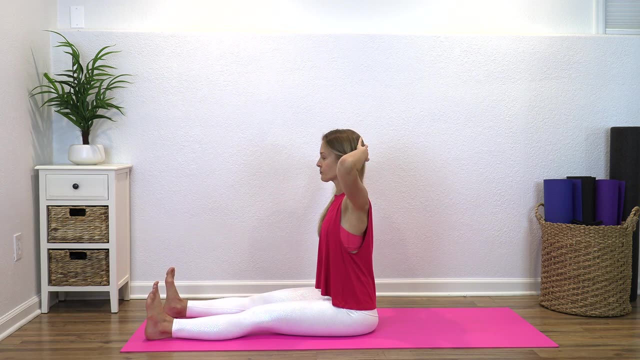 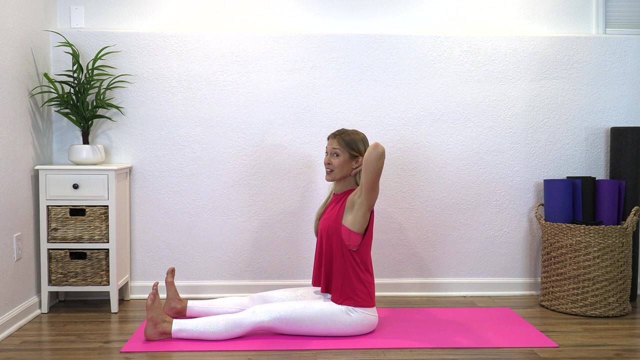 movement up in our thoracic spine. research shows there's a direct connection from our thoracic spine to our pelvic floor. so we're gonna move that thoracic spine hands behind your head, elbows wide, so you're gonna sit up as tall as you can and then maybe find that pelvic floor contraction here and 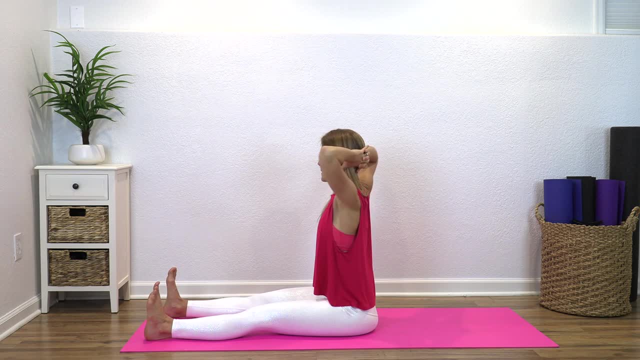 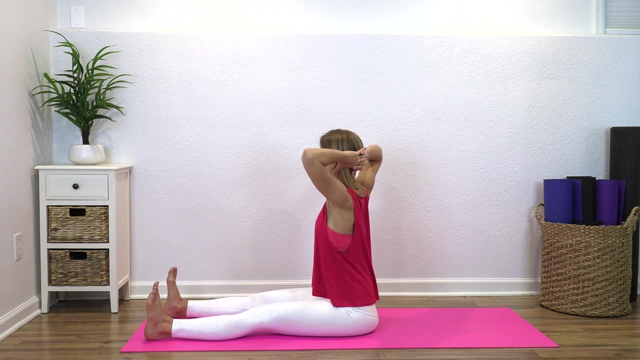 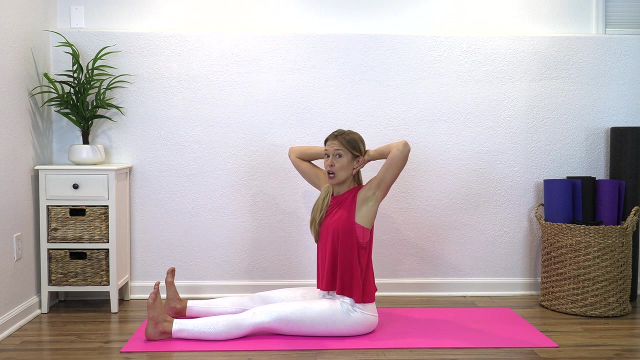 now rotate to your right, center, left, center, okay. so again you're kind of thinking about drawing that bean up and in and then you're trying to get that upper spine moving. so don't be surprised if you feel tight in this position, like you might feel tight. 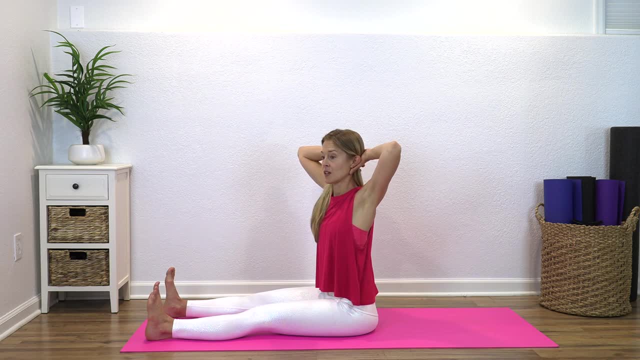 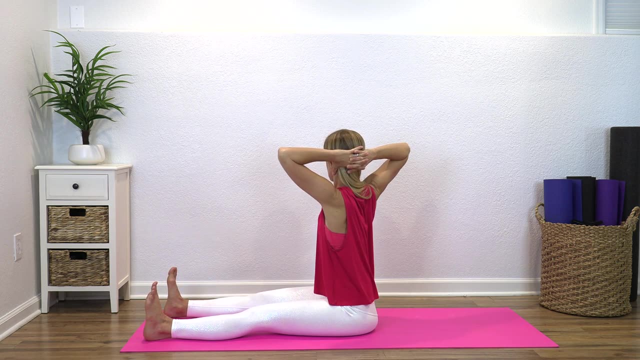 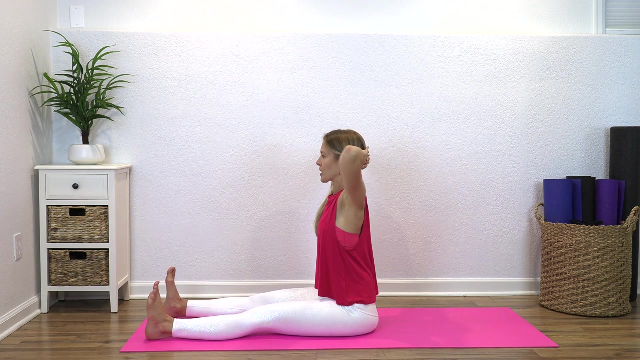 in your hips. you might feel tight in your back, but again, think about sitting up as tall as you can and trying to lift the pelvic floor, even as you're kind of trying to lift your ribs up off of your hips. alright, one more to each side. last, 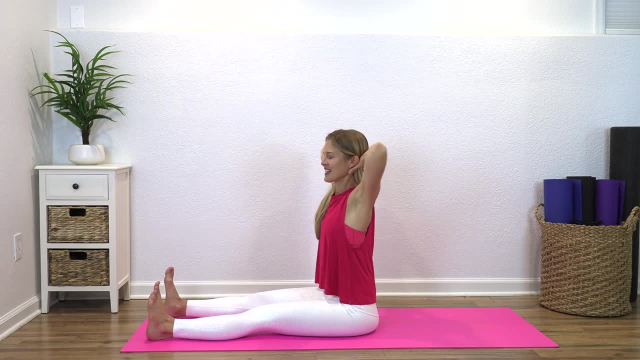 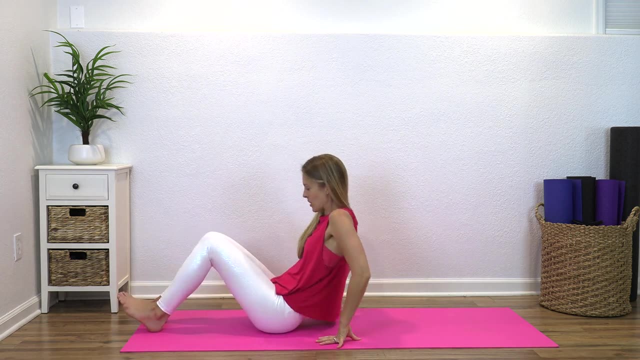 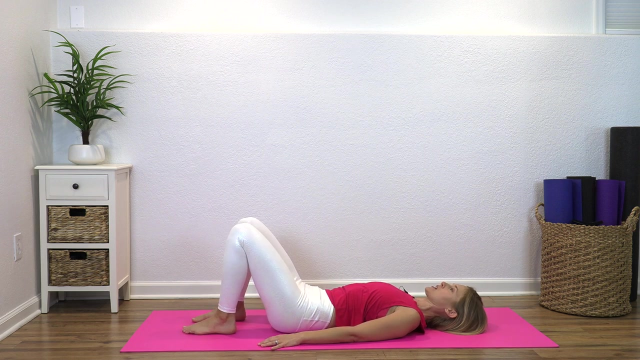 one nice job. hands come down and then lay down on your back. this is gonna be our last thing, so feet are gonna be hip distance apart. arms relax at your sides. take your inhale now exhale. curl your tailbone. roll yourself up one vertebrae at a time. 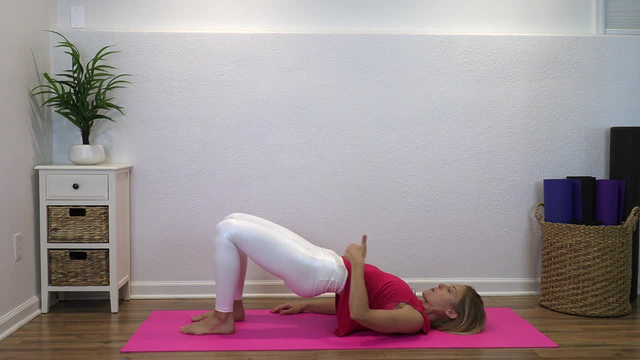 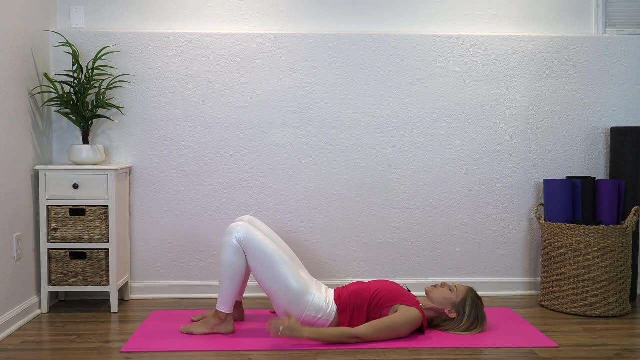 ok, inhale at the top, draw that pelvic floor in, exhale multiplex, dobrow, roll back down. so what we're trying to do now: inhale at the bottom, exhale to do the same thing again. we're trying to get the spine moving. 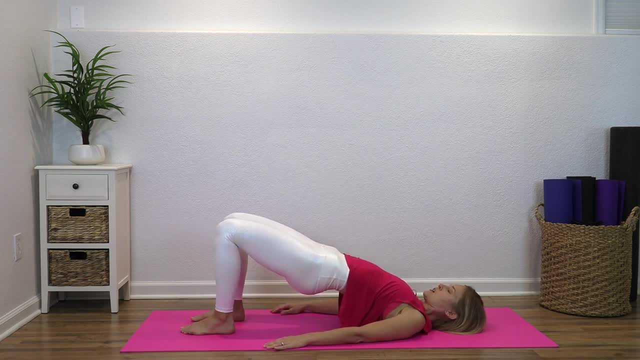 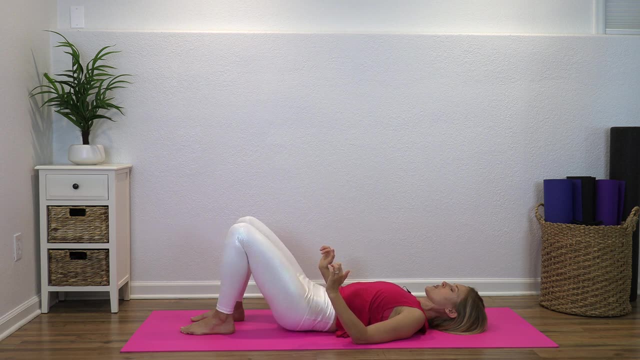 okay, i just had you do some rotation for the spine. now we are trying to articulate inflection and this natural movement and what happens is when there's a dysfunction we kind of lose that. we either really guard in our pelvis, things get tight so we want to try to move and it's 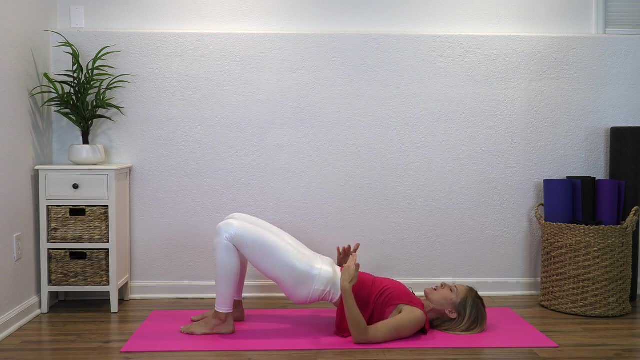 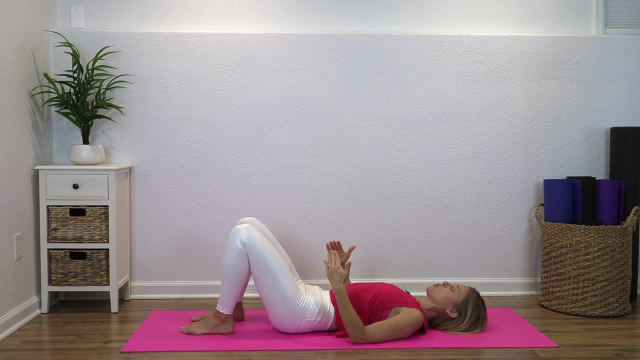 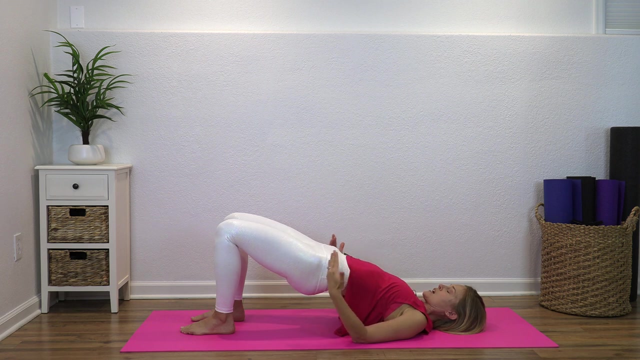 also a nice place to make the pelvic floor feel better, because you're de-weighting it, meaning when you roll up into that bridge you're up against gravity right. so there's not any weight down on the pelvic floor, it's just a little bit more of a stretch. so we're going to do a little bit more of that. 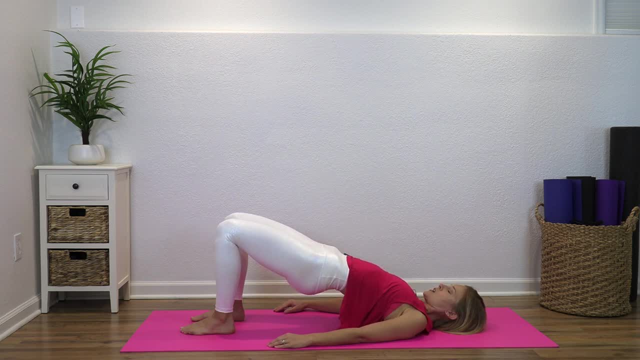 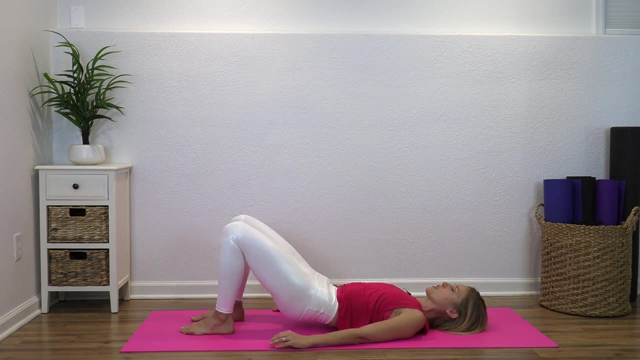 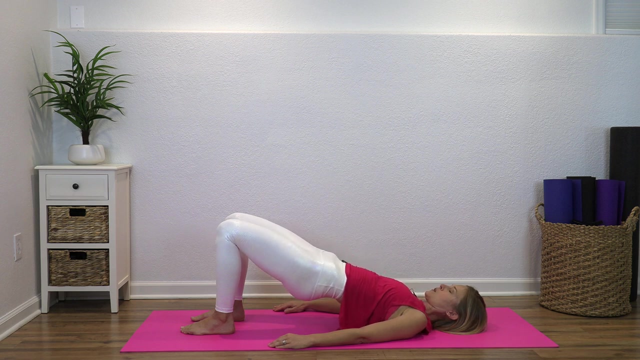 nice job, so here too, you can pull in on the pelvic floor when you exhale. you can inhale, release it, exhale to roll down. what i really want you to focus on, though, is that moving through the spine. okay, just one more of these nice job, so that was about 10.. okay, so you can roll to your side. 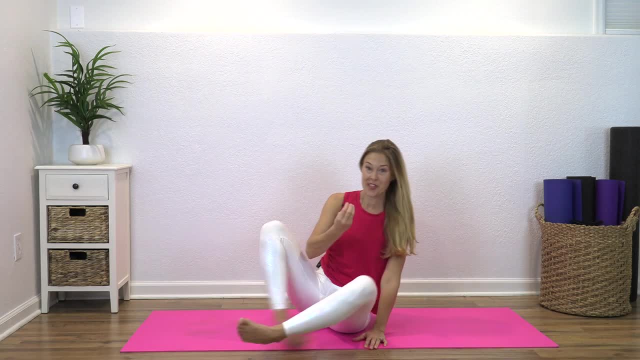 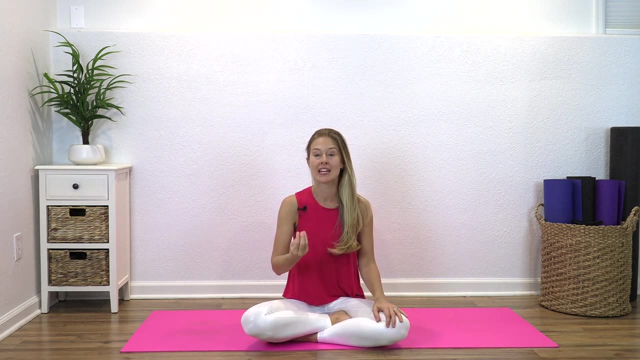 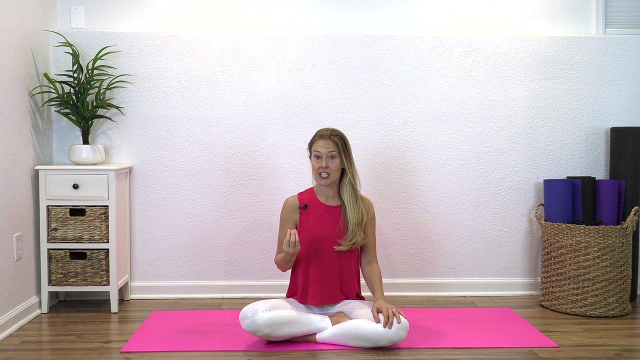 and sit up and i'm going to review all of that. so if you are having pelvic floor issues, if you've been told you need to help strengthen, if you've recently had a baby, if you've recently had a hysterectomy, you can start all of these. you want to do it every day for at least 30 days, so just keep.